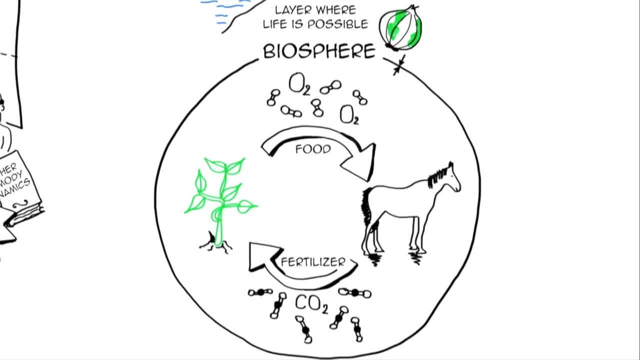 animals produce fertilizer and CO2, carbon dioxide, which are used by the plants, and we have a cycle that is well balanced. This is a very quick cycle. We eat every day and we breathe every day. We eat every day and we breathe every day. We eat every day and we breathe every. 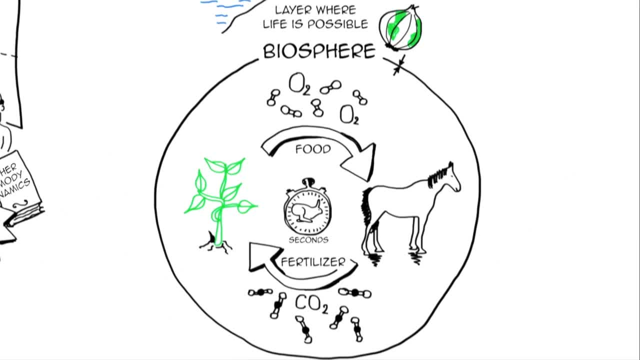 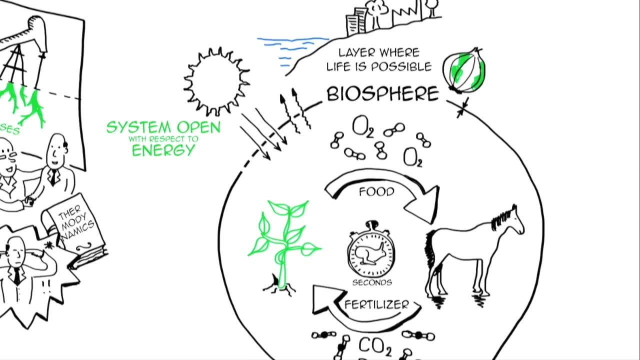 second, and it works well. Then they agreed on the fact that this system, the biosphere, is open with respect to energy. This means that energy from the sun comes in and radiations come out. This is also known as the first law of thermodynamics. They also agreed on the fact: 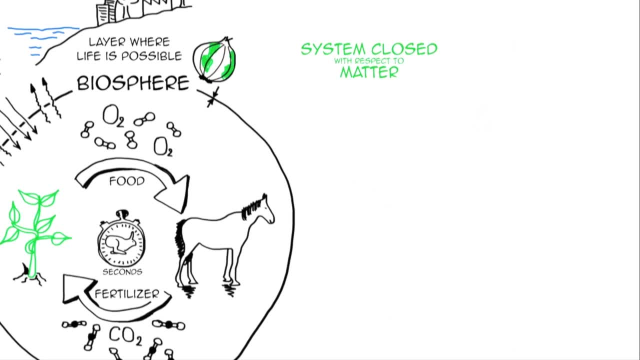 that this system is closed with respect to matter. So maybe you remember this very famous phrase from Lavoisier that says nothing is created, nothing disappears. And so they agreed on the fact that everything is only transformed. This is also known as the law of conservation of matter, And 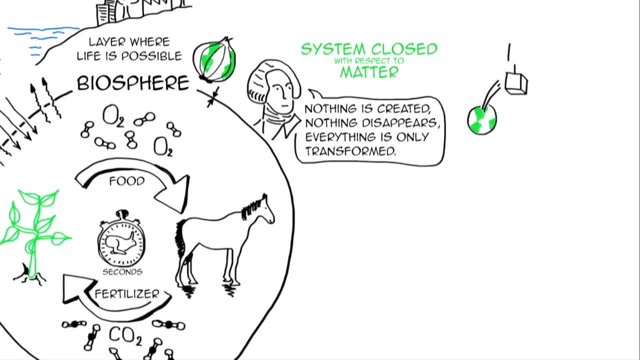 it means that, except for a few satellites and meteorites, all the matter that was on Earth 4 billion years ago is still here today. It has changed form and the molecules have reorganized themselves, but it is still the same matter. The other thing that comes with this is that 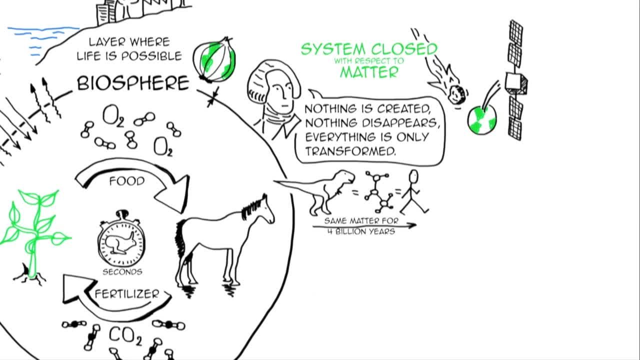 everything has a tendency to disperse. For example, take an iPhone and wait for a million years to see if it can disperse, And if it can disperse, then everything has a tendency to disperse. For example, take an iPhone and wait for a million years to see if it can disperse, And 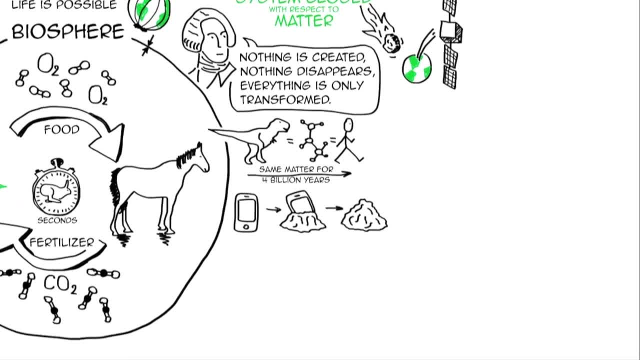 if it can disperse, then everything has a tendency to disperse. And if it can disperse, then everything has a tendency to disperse. And if it can disperse, then everything has a tendency to disperse. It's very likely that you will get a pile of dust. Take a pile of dust and wait for a million years. 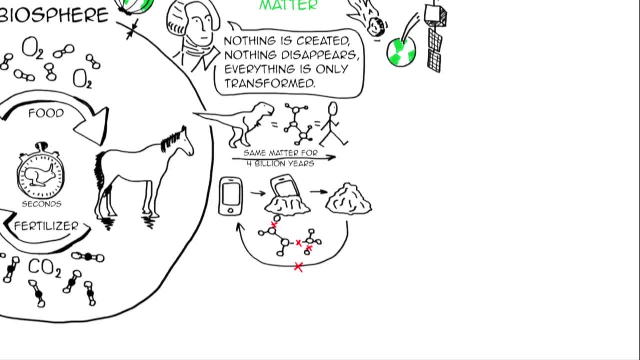 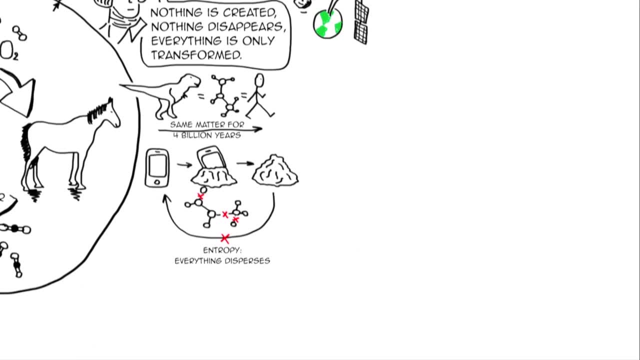 you will never get an iPhone. It works only in one direction. This is also known as the second law of thermodynamics, the law of entropy. So if everything disperses all the time, how is it possible that we live here in such a beautiful world with beautiful nature, cities? 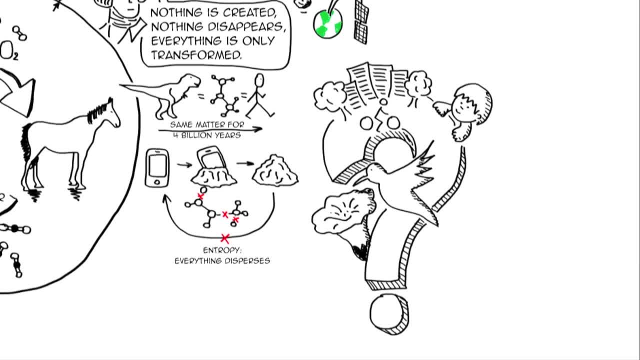 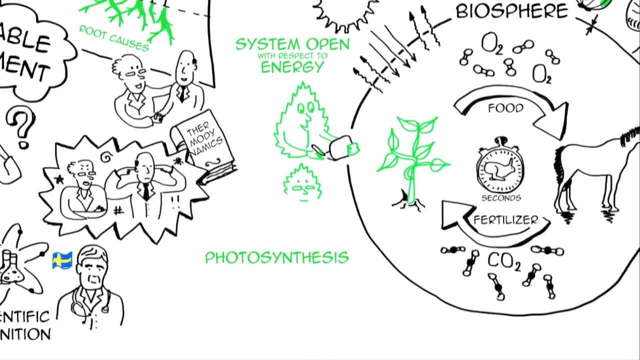 people, flowers and so on. Well, this is what photosynthesis does for us. Photosynthesis pays the bills. Plants have the capacity to use the energy from the sun in order to produce oxygen and sugar using carbon dioxide and water Photosynthesis. 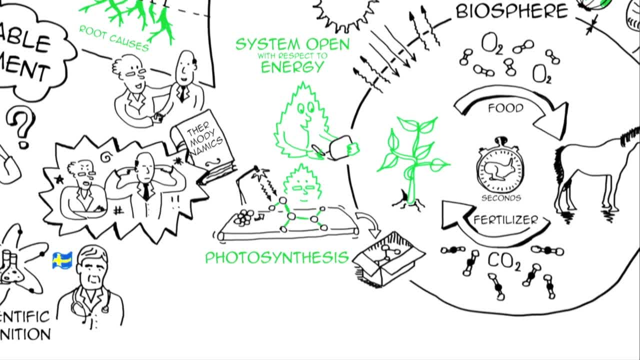 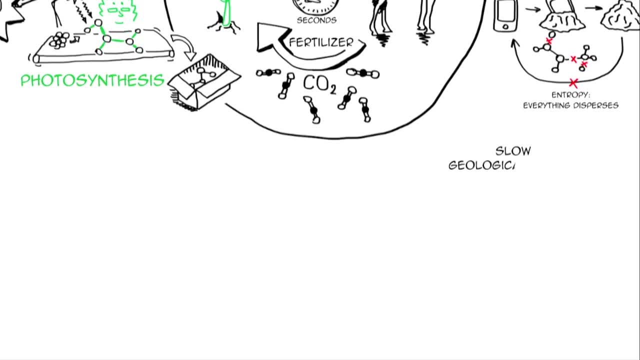 reorganizes matter and creates new structure. The group of scientists also agreed on the fact that there are other cycles, very slow geological cycles, that bring matter from the lithosphere- that we also call the Earth's crust- to the biosphere. 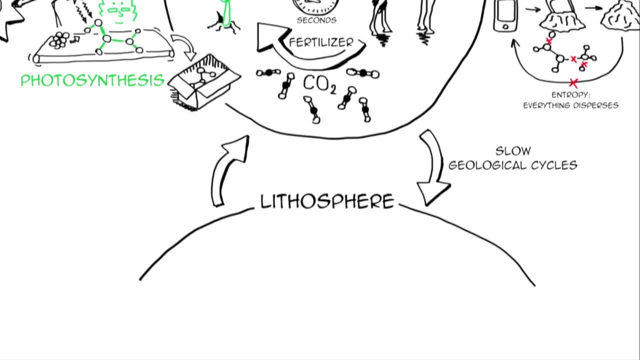 And these cycles are also very well balanced. Some matter moves from the Earth's crust to the biosphere through things like volcano eruptions and weathering, And just about the same amount of matter goes back from the biosphere to the Earth's crust via things like mineralization. 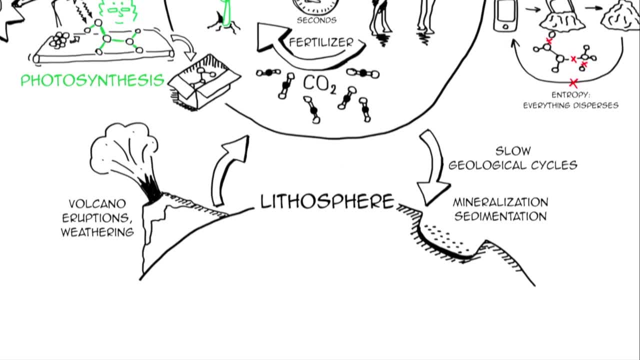 and sedimentations, And all this is very well balanced. These cycles take millions of years, they are very slow, unlike the previous ones, and they also work well. Here's what the scientific community agreed upon. This is the world we live in, So what? 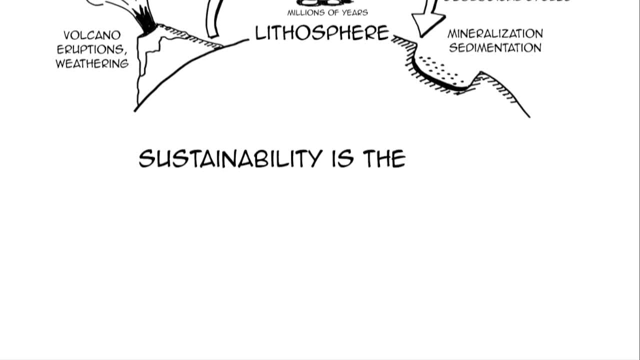 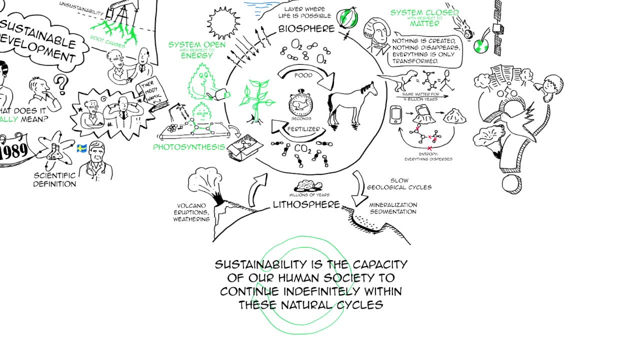 is sustainability? Well, it's actually the capacity of our human society to continue indefinitely within these natural cycles, And sustainable development would be a development towards this state of sustainability. So you may be thinking: well, this does not exactly tell us what to do on Monday morning. 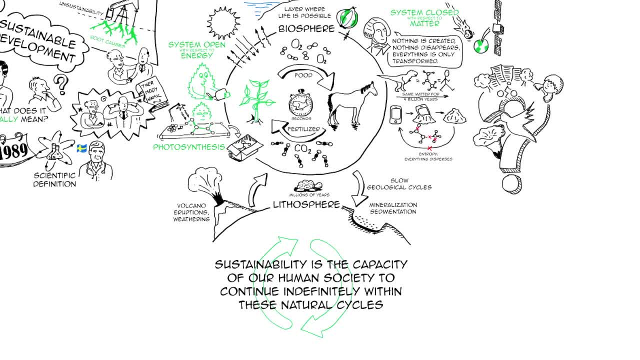 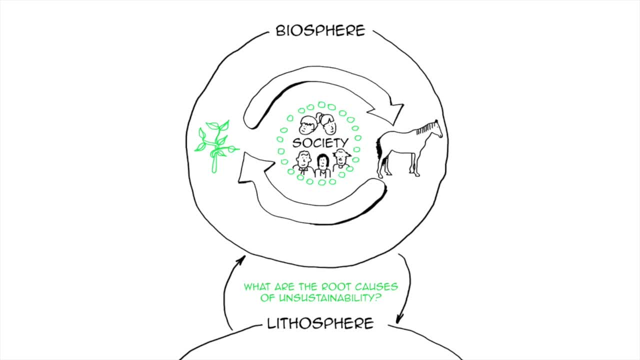 either. That's right, But it made it possible for our group of scientists to look at the things that we do to improve our lives. So what is sustainability? Well, it's actually to interfere with these natural cycles, And they found four root causes of unsustainability. 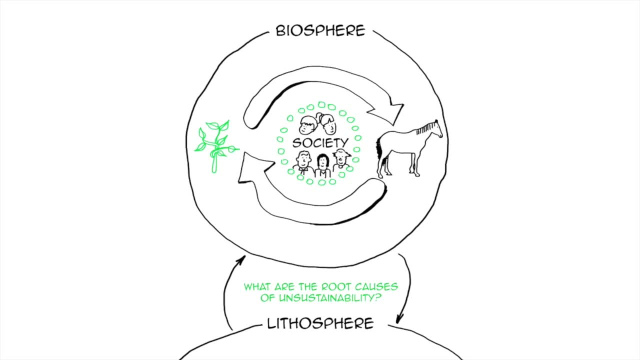 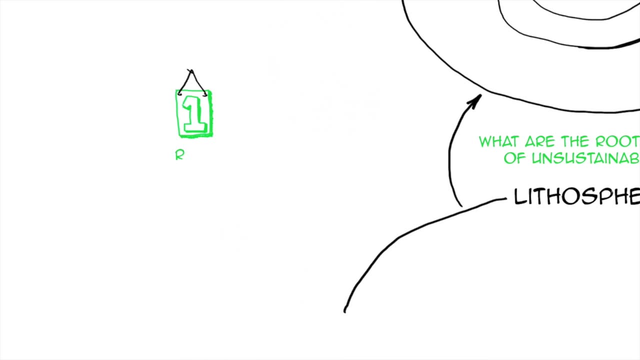 And these are the four things that we need to stop doing to be sustainable. They're all equally important, They're all necessary and sufficient. The first one is that we extract large flows of materials from the Earth's crust, the lithosphere. These materials are things like oil, like natural gas, heavy metals, etc. that are 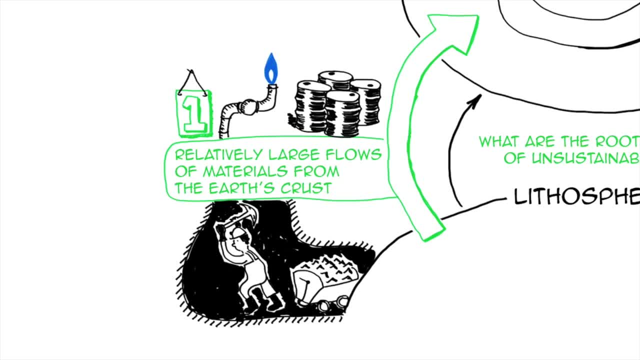 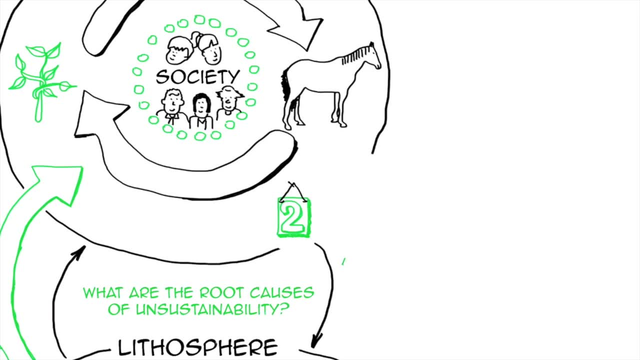 rare in the biosphere And that we extract in such large quantities that they accumulate and nature cannot cope. The second one is that we create in our society substances that accumulate in nature. We create chemical compounds that nature takes a very long time to break down. But we also create. 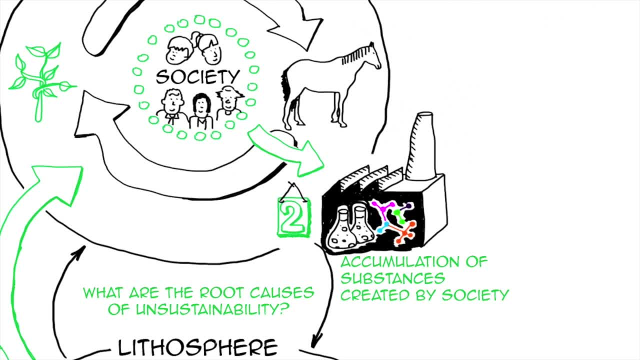 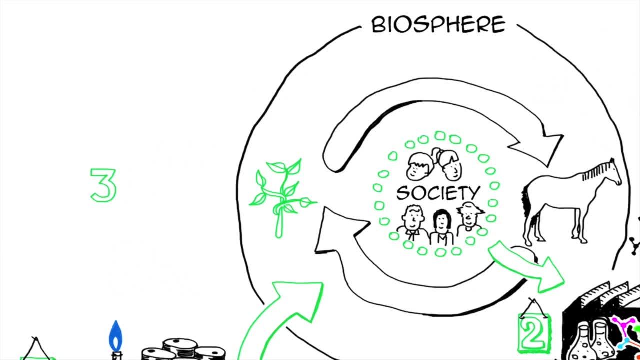 substances that already exist in nature, like carbon dioxide, for example, but in such large quantities that they accumulate and nature cannot cope. The third one is that we physically inhibit nature's ability to run the natural cycles. How do we do that? Well, for example, by chopping trees at a faster rate than they can grow.